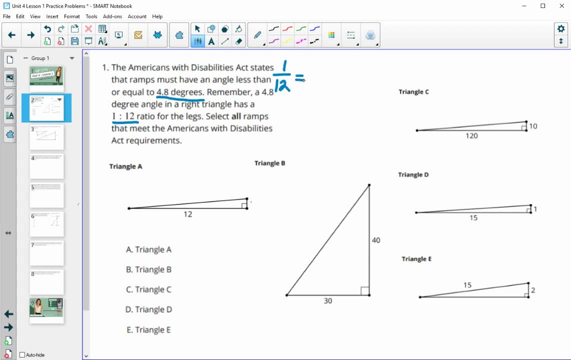 to 12.. So I just looked at a ratio of 1 to 12 in decimal form to help me figure this out. And so 1 over 12, as a decimal, is equal to 0.083.. So we can kind of take a look at these and the looks like the. 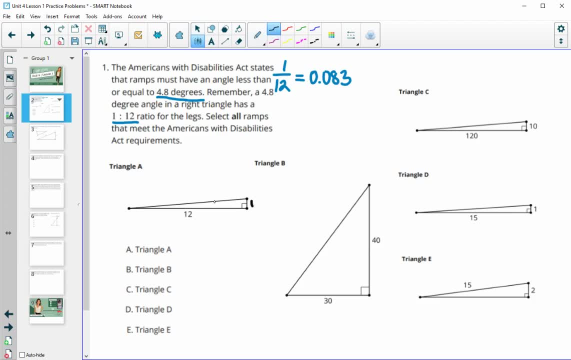 one got cut off here, So this one is supposed to say 1.. So when we look at this ratio in triangle A the ratio is 1 to 12.. Well, we know that's equal to 1 to 12. So triangle A is definitely. 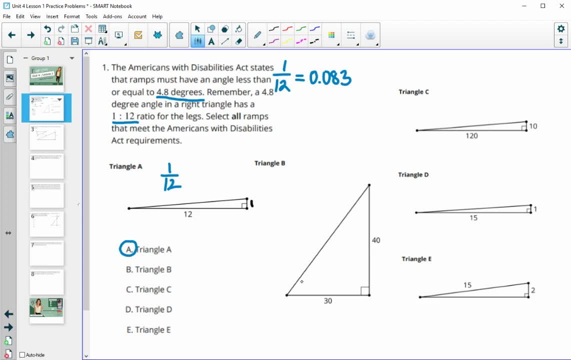 in compliance. Triangle B, and remember this is the ratio of 1 to 12.. So triangle A is definitely in compliance. Triangle B, and remember this is the ratio of 1 to 12.. So triangle A is definitely in compliance. Triangle B: 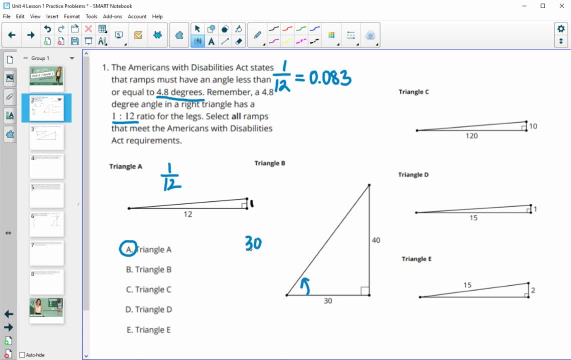 is the angle right here. So we're looking at this steepness, So we're looking at 30 over 40. And this one simplifies to three-fourths, which is way larger than 1 to 12.. So we know that this 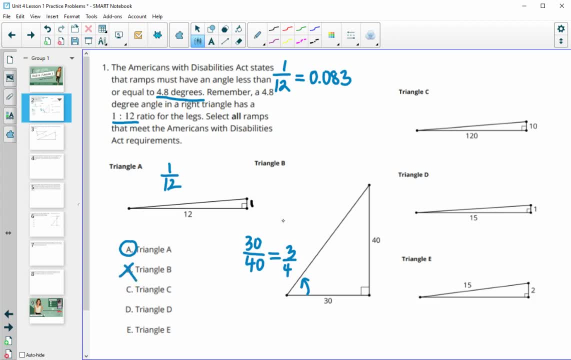 does not work. You could also divide this and get that it's a decimal of 0.75,, which is a lot more than 0.08.. So that is way too steep. Triangle C is a ratio of 10 to 12.. So triangle C is a ratio. 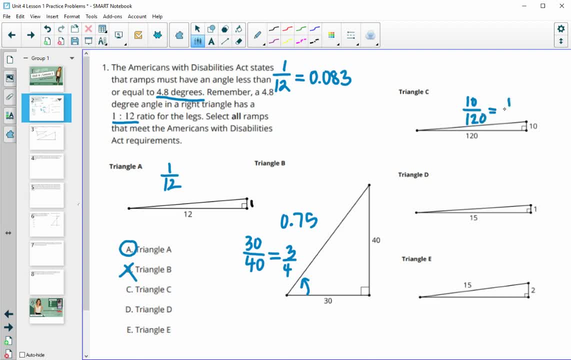 of 10 over 120.. And if you simplified that by dividing each by 10, it would be 1 over 12.. So that's equal to the ratio, or equal to a 4.8 degree angle. Triangle. D is 1 over 15.. And 1 over 15. 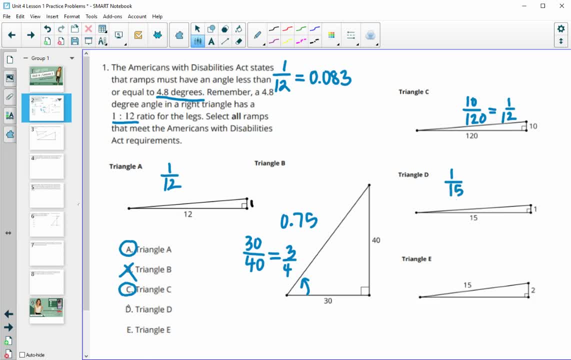 is less than 1 over 12.. So this one is good. And if you are struggling with that and you divided this down, 1 divided by 15. Is 0.066.. So that is less than the 0.08 requirement. So that's going to show you it's good. 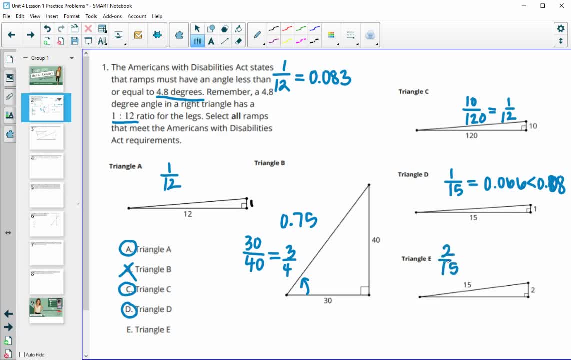 also, Triangle E is 2 over 15. And so then this decimal is 0.134.. And that is not less than the 0.083 requirement. So triangle E is 1 over 15. And so that is less than the 0.134 requirement. 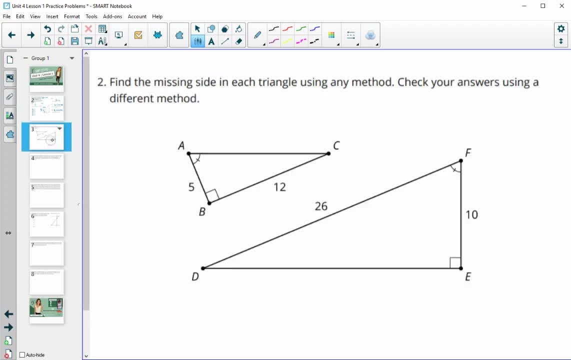 This is not that good, because if you are certain second is less than first, you're going to have to adjust that to 1 or 2.. to get it back to where the residual vastness would be: So triangle E is 2 over 15.. 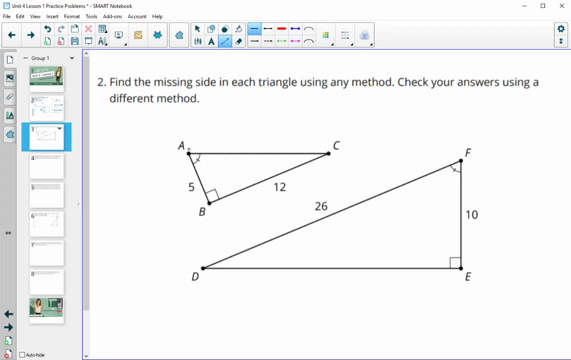 So triangle E is 2 over 15.. And so you can get acolon. So triangle E is two over 15.. And so the second one is equal to 0.双 If you divide the three in. So we would say: AC squared is equal to 5 squared plus 12 squared and solve that way. 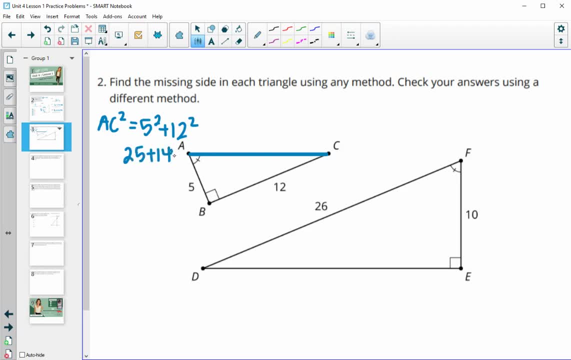 So we've got 25 plus 144, which is 169.. So that's AC squared, And then we could square root that and we would get that AC equals 13.. So that's one way to do it. Another way would be to do proportions. 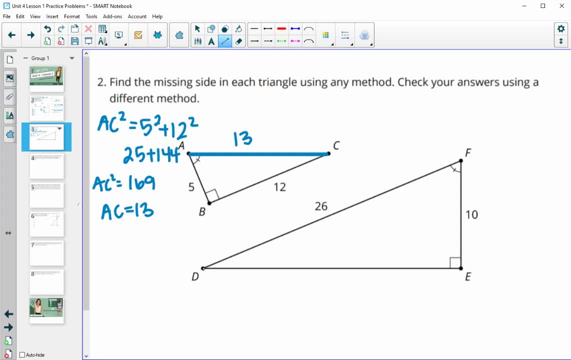 So we could have found this one by comparing similar sides in the other shape. So this is the hypotenuse that's missing in this one. And then we could compare two other similar sides And we see that this one has the shorter side with the right angle. 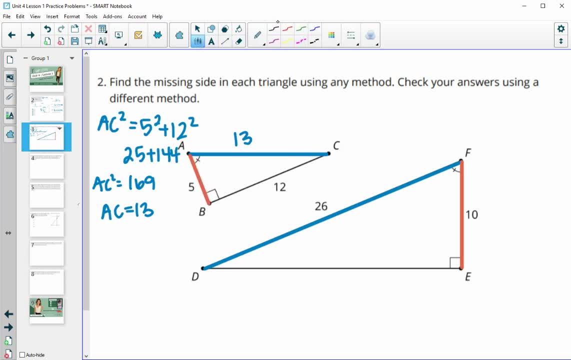 And so we could compare that here. So we could have done a proportion to find this. So, pretending that we didn't know this yet, we could have set up a proportion That compared 5 to 10. And then compared the hypotenuse here, AC to 26.. 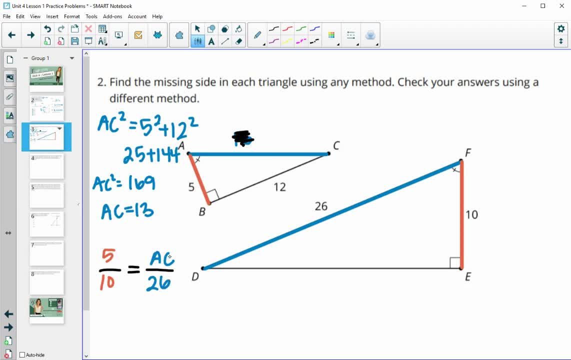 And so you can see that 5 times 2 is 10.. So what times 2 is 26?? So we would have gotten 13 that way. If you noticed there with kind of a scale factor idea, you could also cross, multiply 26 times 5 and then divide by 10.. 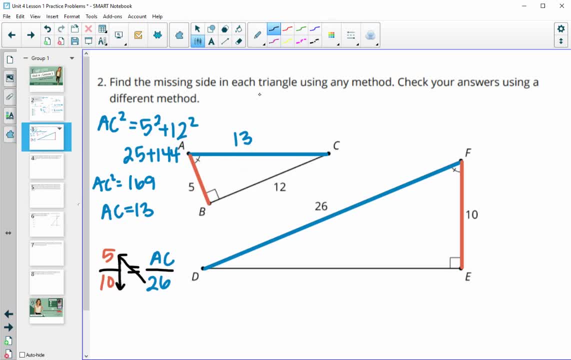 And that would have gotten you 13 as well. So then, for this final missing side over here, I'm just going to do the scale factors, because it's quicker for me. So when I'm looking at this one compared to this one, so we can see that this triangle is just two times larger, right? 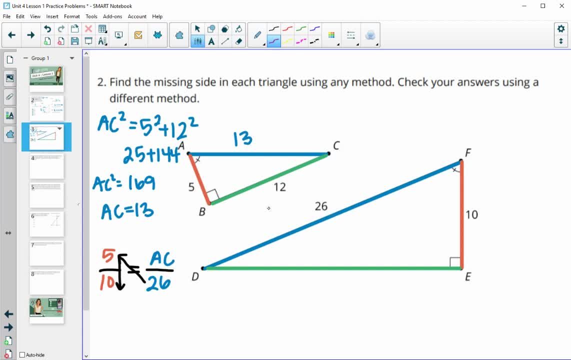 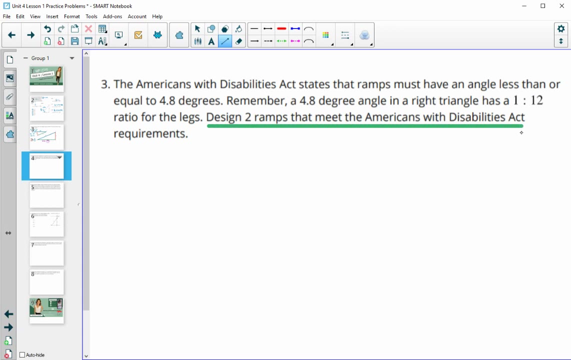 So 5 times 2 gives us 10,, 13 times 2 gives us 26.. So this side is going to be 12 times 2, which is 24, for that one. Number 3 asks you to design two ramps that meet the ADA standards. 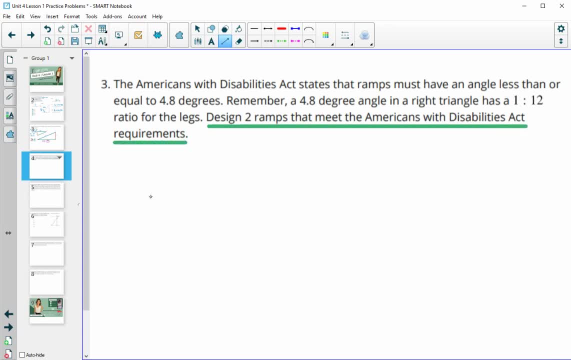 So meaning that the ratio of the height to the length needs to be less than or equal to 112.. So you can do kind of anything you want. You just got to make sure that when you compare the measurements that you used, that they meet the ADA guidelines. So if I was looking at this one here, you know I don't want to do it, you know I don't want to do this. Like I said, I don't want to do it. I'm sorry. I'm sorry. It's just I don't want to do it, So I'm sorry. I'm sorry, I don't know if you have any other questions. I'll move forward to the next slide, Thank you, Thank you, Bye-bye. 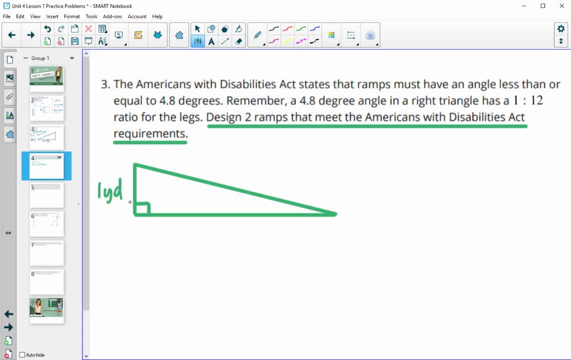 I do this one and I say this is one yard. this one has to be at least 12 yards. So if I put 13 yards, that's going to be fine, because one over 13 is less than the 1 12th requirement. So there's. 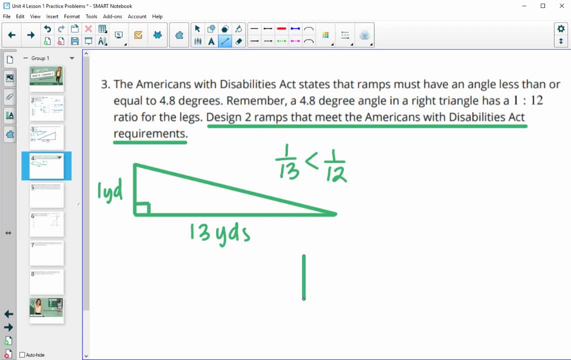 one that works. You could do many other things, So if I wanted, so that one's in yards, maybe I'll do feet for this one. So if I said that this one is three feet tall, so three if my top number is. 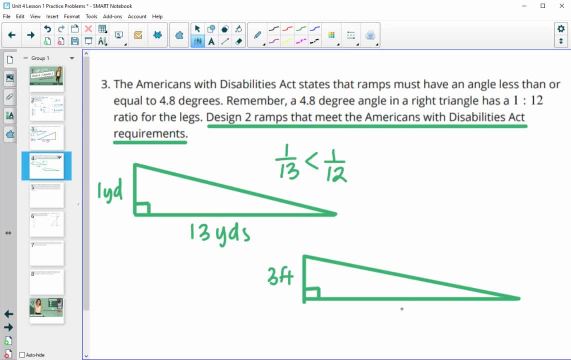 three, 12 times three is 36.. This has to be at least 36 feet long. So if I put 40 feet down here, that's going to be fine, And you could also then divide three by 40 to figure out that that's less. 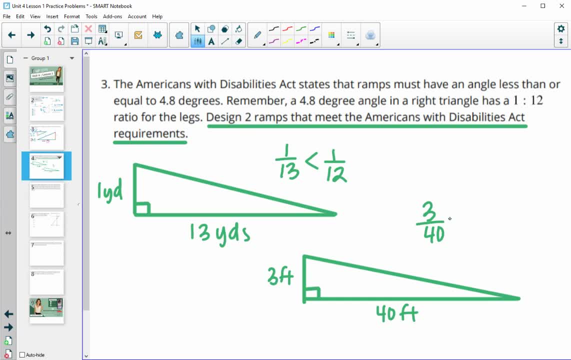 than one divided by 12.. So three divided by 40 is equal to 0.075.. And, if we remember, one divided by 12 was 0.083, and that is less than that. But plenty of different options that you could do for this one. 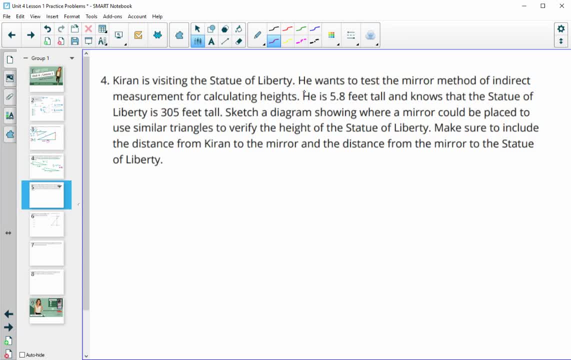 Number four: Kieran is visiting the Statue of Liberty. He wants to test the mirror method of indirect measurements for calculating heights. He is 5.8 feet tall and he knows that the Statue of Liberty is 305 feet tall, So he has a diagram showing where a mirror could be placed to use similar triangles. So if we kind, 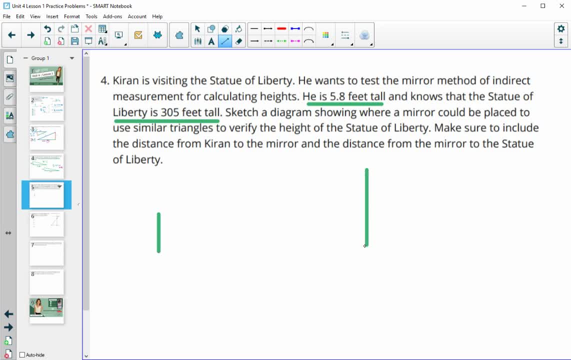 of draw Kieran here and then we draw the Statue of Liberty here. okay, then the ground will connect them And we're going to try and figure out where the mirror would need to be placed in order for this to work. So let's fill in these heights So we know that Kieran was. 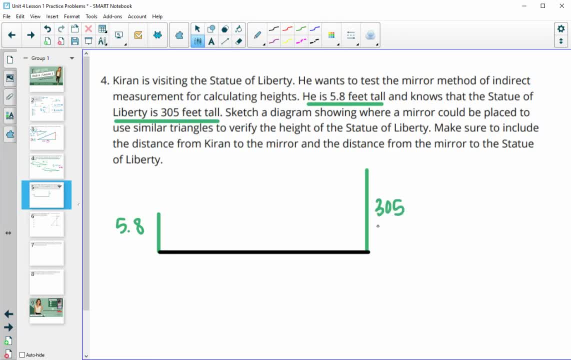 was 5.8 feet tall and the Statue of Liberty was 305 feet tall, Then I'm just going to sketch these in. It doesn't really matter on my drawing necessarily where they are, but we got to figure out something to say for this. So we're trying to figure out this placement. 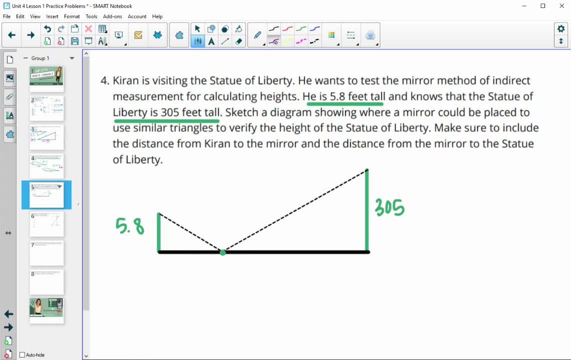 So remember that we want it to be proportional, And so you know that we have to figure out what scale factor takes this to this. Okay, so our K value is going to be 305 divided by 5.8.. And that is, 305 divided by 5.8 is 52.59.. So this is our scale factor. So, no matter what, 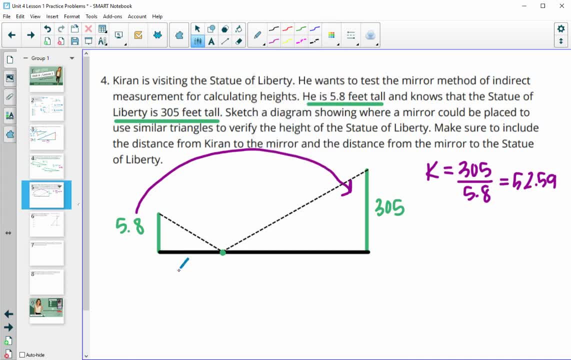 measurement you put here, however long this is, this number needs to be 52.59 times that number. So if? and it doesn't tell us how far apart these are, So it doesn't tell us how far Kieran is standing from the Statue of Liberty, Otherwise we could divide. 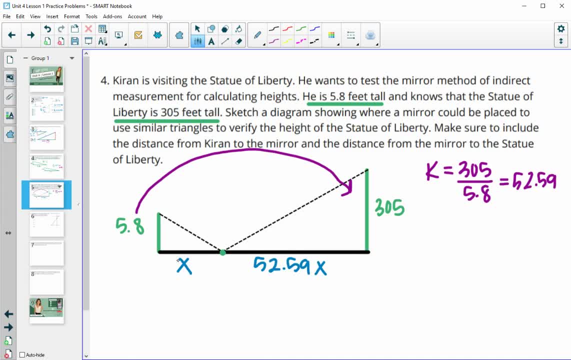 this out, But it doesn't say that, So you can just pick a number here. So if I said, um, let's say, Kieran is standing um 25 feet, Okay, He could be 20,, 25 feet from the mirror. If this is the case, then we would do 25 times 52.59.. And um, so it. 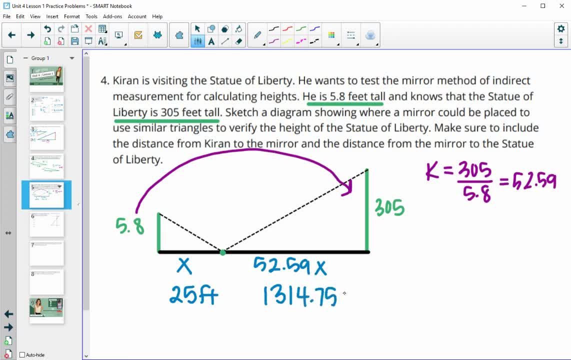 would be 1,314.75 feet away from the Statue of Liberty, So this first part would be 25.. This second part would be 1,314.75.. That would be something that would be fine, And again, you can do other things. So we're trying to figure out how far apart these are. So we're 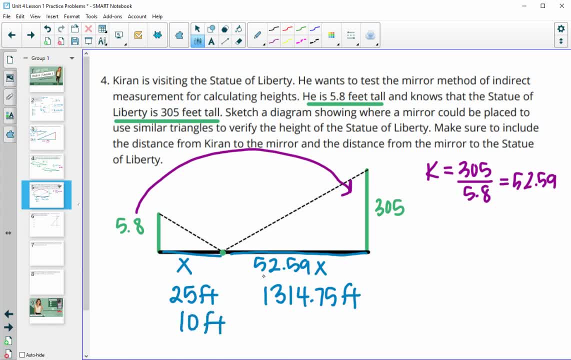 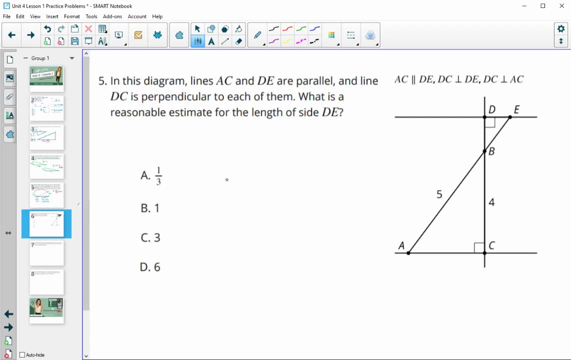 like if you put 10 in here. if you said that this first measurement was 10,, then the second one would need to be 52.59 times 10, which is 525.9 feet. So you just have to make sure it's in that same scale. Number five in this diagram, lines AC and DE: 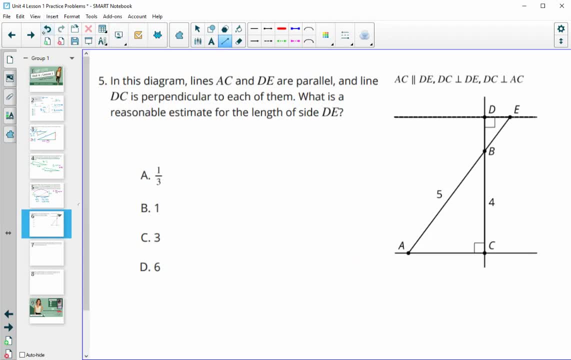 are parallel And um line DC is perpendicular to each of them. What is a reasonable estimate for DE? So we're looking for a reasonable estimate for this one. So we need to have this to kind of be able to compare. And so we see that this is a right triangle down here with a. 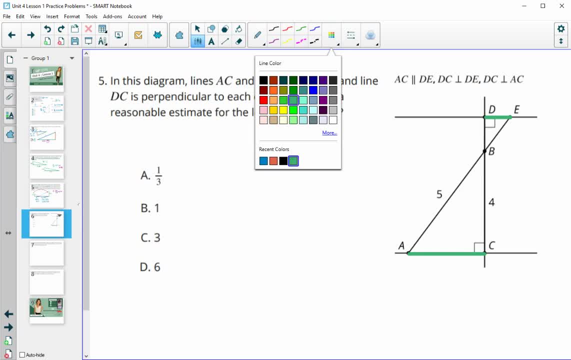 hypotenuse of five and a leg of four. So maybe you've used this one enough to know that this is going to be three. Otherwise you can do the Pythagorean theorem quickly, um, to figure that out. So five squared equals AC. 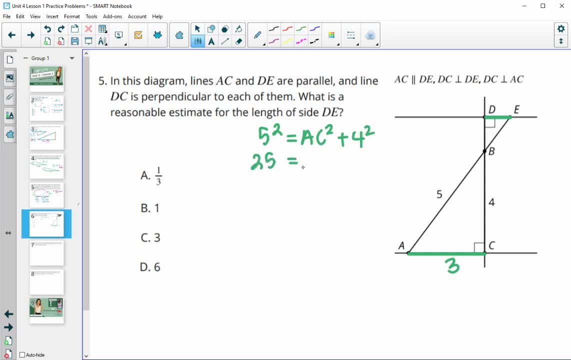 Squared plus four squared, So you'll have 25 equals AC squared plus 16.. Subtract 16 to get nine equals AC squared, And then um square root that. So now we're looking for things that make sense. um, for the length of DE. So it's obviously getting smaller, So it's not going to. 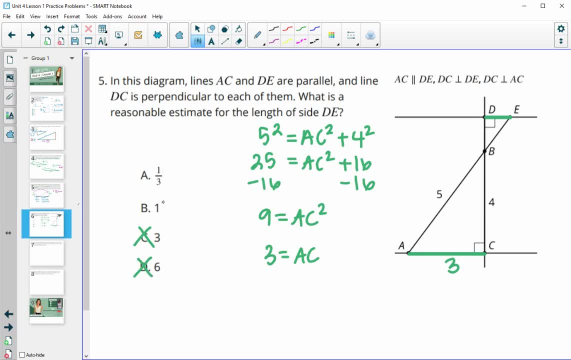 be the same size or larger. So it's going to be one of these And, um, if you kind of take a look here, let me change the color of this. But so if I took this segment and just looked how many times, it kind of fits in here. So one, two, about three times, right? 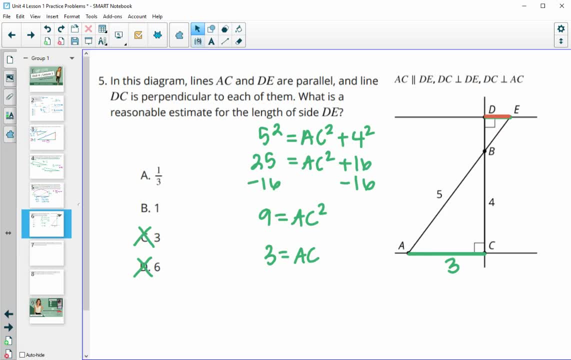 So this length here is going to be one third of the original. Okay, So this is going to be one third of this measure. So this is going to be three times one third, which is one. So that would be a reasonable estimate. 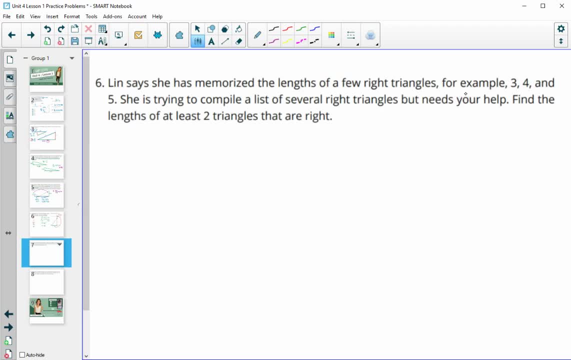 Lynn says she's memorized the lengths of a few right triangles, So the one that I just talked about, um, a three, four, five right triangle. She's trying to compile a list of several right triangles, but she needs your help, So give her a couple more. So she has three, four, five. 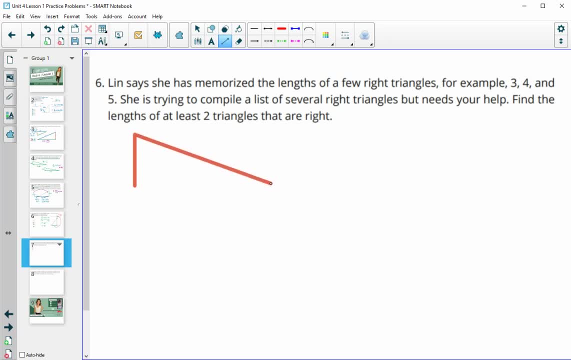 Um, another fairly common right triangle, Pythagorean triple, where all of the sides of the whole numbers is a five, 12,, 13. So this is 25 plus 144 is 169. So that one works Um. 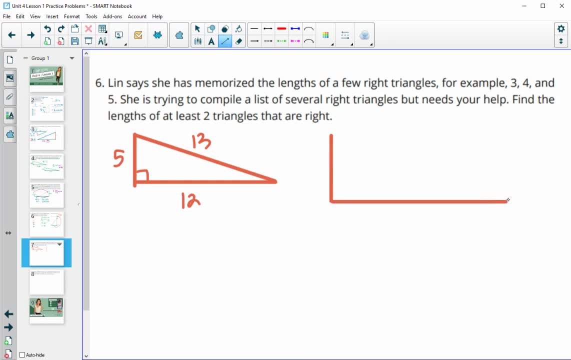 another one is a seven 24, 25.. So seven 24, 25.. So if you square these out, seven squared is 49.. That equals 625, which is what 25 squared is. So there's two Um. another pretty common one is eight. 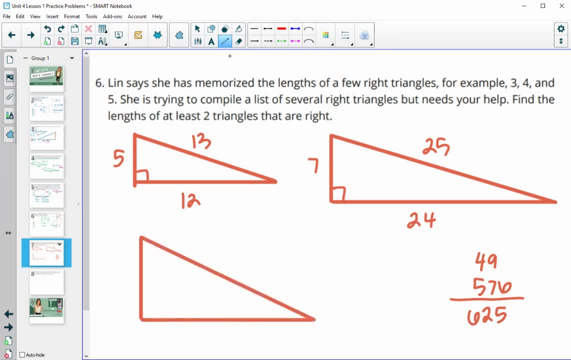 15, or sorry, Yeah, Eight, 15, 17.. So eight and 15 for the legs and 17 for the hypotenuse. So eight squared is 64.. 15 is 225.. So if you add together is 289, which is what 17 squared is, And I'll just write this one out too. 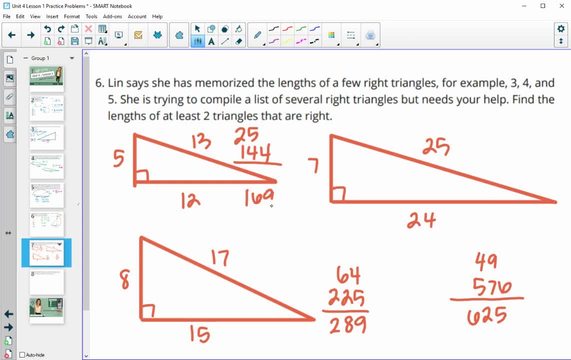 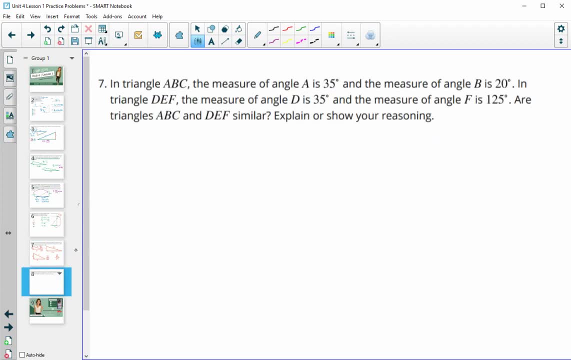 was 25 and 144, which totals out to 169,, which is what 13 squared is. And then, finally, number seven says in triangle ABC, the measure of angle a is 35 degrees, The measure of angle B is 20 degrees Um. 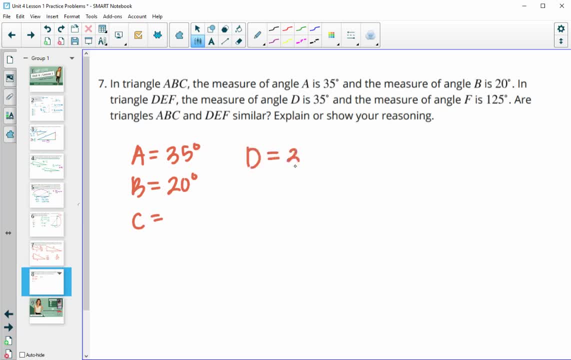 and then number six says in triangle ABC, the measure of angle B is 20 degrees Um. and then number seven says in triangle B is 20 degrees Um. and then it says in triangle DEF, the measure of angle D is 35 degrees And the measure of angle F is 125 degrees. Are they similar? Explain or show. 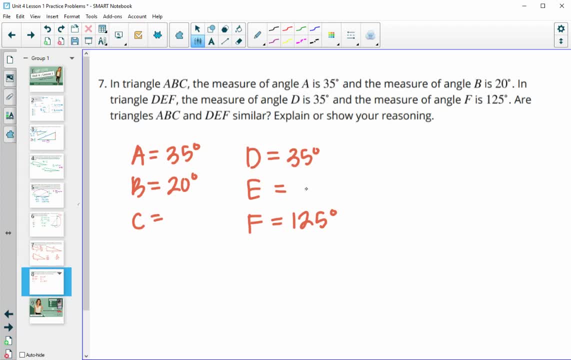 your reasoning. So we just need to find one of these two missing measurements so that we can see if they have two angles in common, Cause we already see that they have one angle in common. So we'll take the triangle sum, which is 180 for all three.